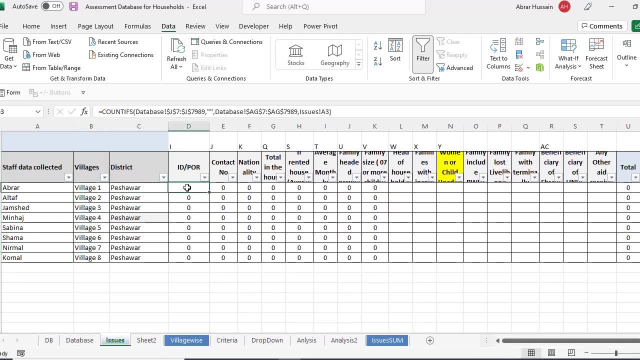 Villages, Districts, So that if there is an error, so you might be able to see whether that error is, in which staff member data are, in which village data and you just go there and clean that. So I have brought here all the columns against which the data has been entered. For example, here you see from ID: 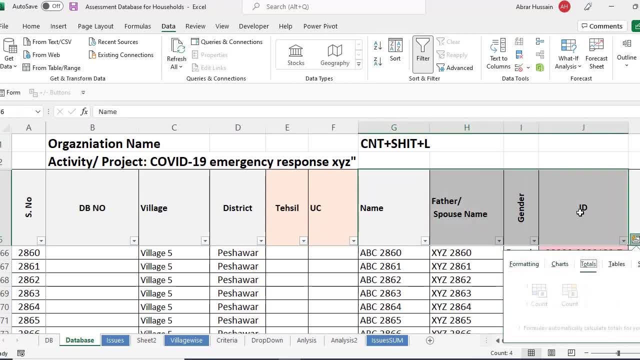 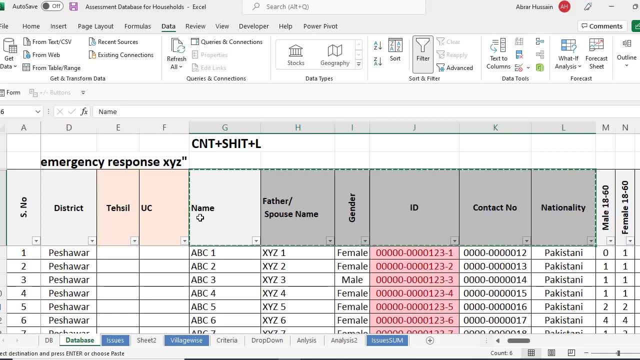 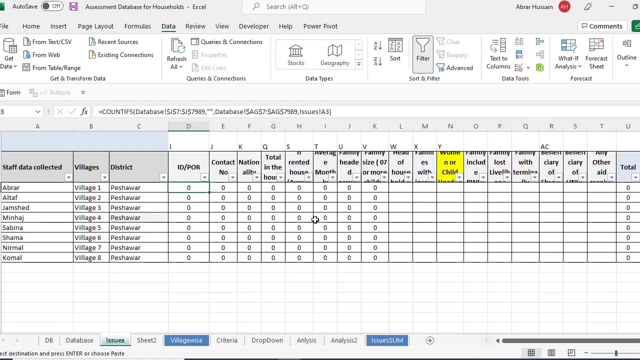 from name to ID. You can take all these columns. For example, if I want to see whether there is any blank info, I can take all these columns. So I can take all these columns. So I can take all these columns, So I will copy these and make an issue sheet and pass those columns here, And then what I will do I 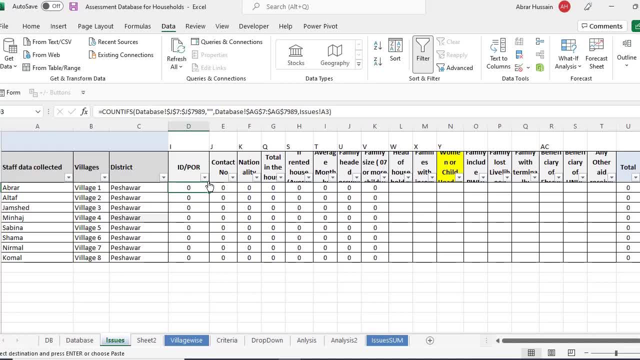 would go to the database and analyze the information. For example, I am going to see whether there is any blank information in the ID card so that I can simply do with count if and submit the methods that I have already explained in previous session, But here I will do them again. Now you see, you can do this cleaning by 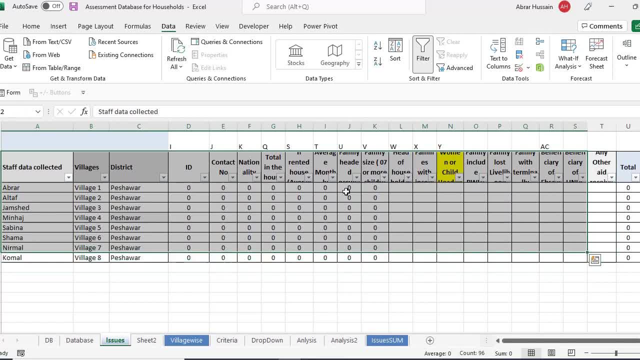 filtering also. but if you do it like this, you can share a table and analysis with people that how much information is missing in id, how much is in contact number, what is the analysis, so you can share a detailed, in-depth review if you don't want to do cleaning with this, so you can go to the next. 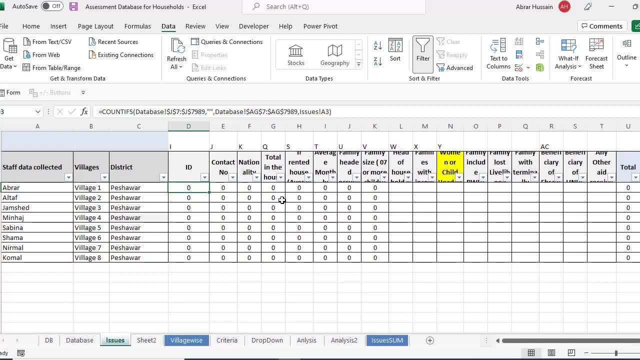 chapter. you can just click in the description, because i have given the chapter's name also, and the disc that is available in the description are in the lower side of the video. so, uh, here what i would do. i, i have used the formula count. if then i go to the database, 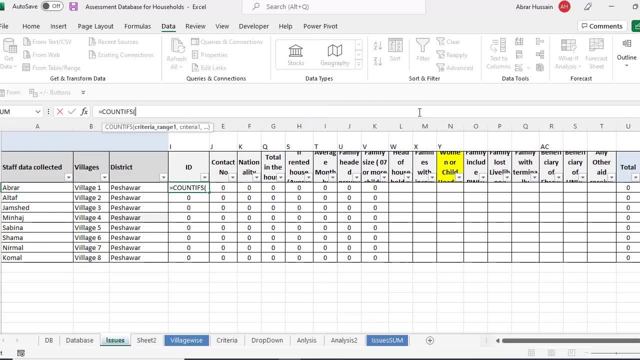 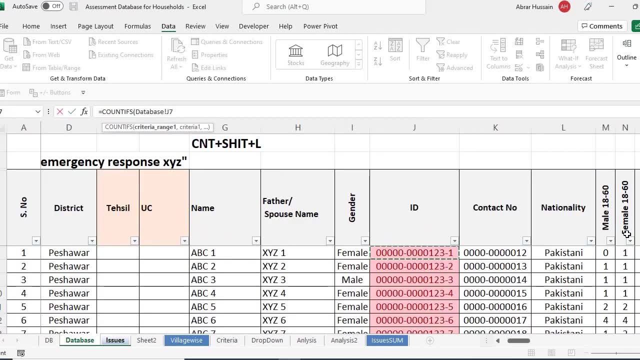 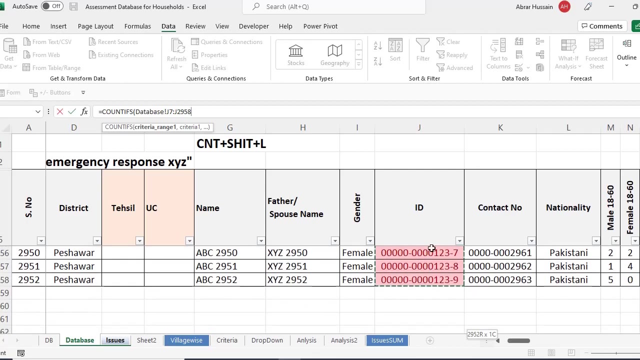 okay, and what i see. look, count ifs. i go to the database and which column: id card. i just select it from start to the end. how i did it? click in the first row and then control, shift down arrow, so it will select the whole database till the end, only that column. so i have selected the id. 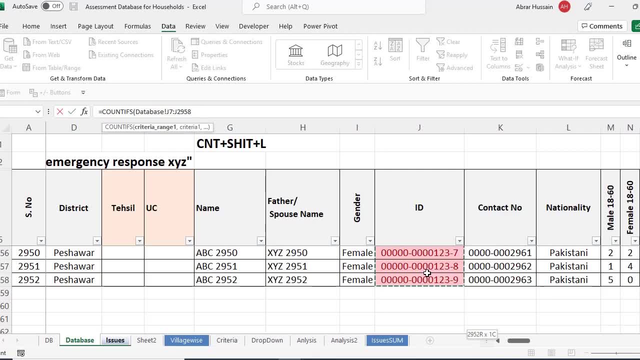 column, then i will apply dollar, as i mentioned before in my previous video. dollar to lock this range. then comma, against which i am going to? against which? against blank, if there is any blank. so for blank, what is the formula? call it inverted comma. start inverted commas close. 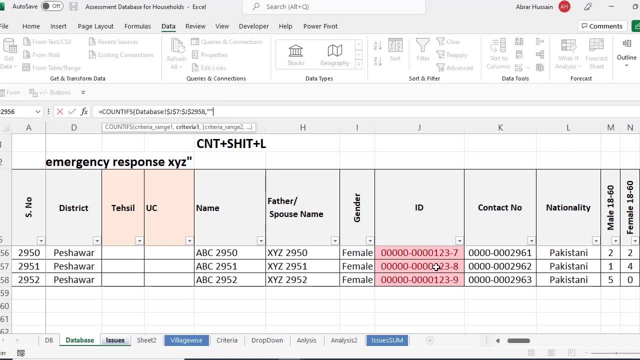 and these are also cut quotation mark. okay, so this means that it will count all the information that is blank, inverted commas, blank and against which i also want to see it. uh, exactly against a staff member or against anyone. so you can apply that criteria also. and then the simple method i. 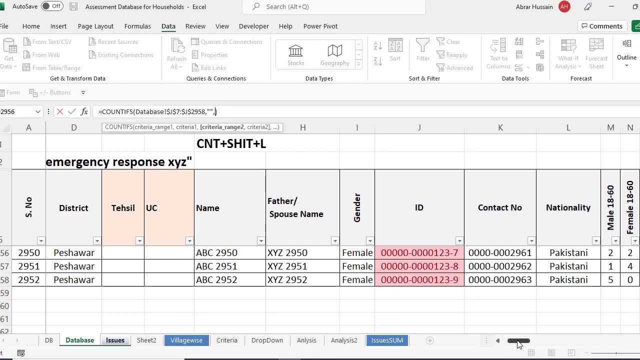 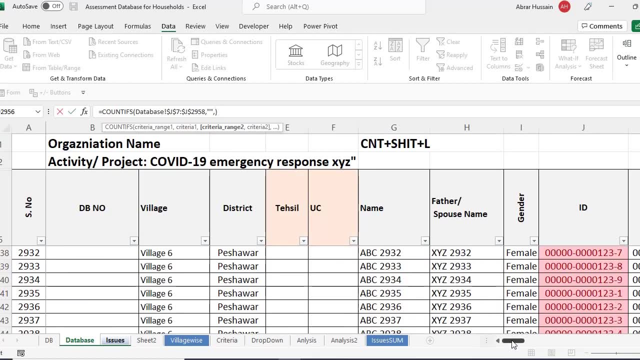 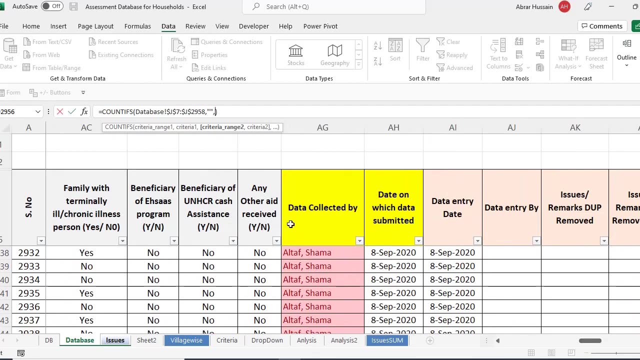 have already explained in the count ifs formula that then you would have to: if you want to see this by villages, so you will select the village column. if you want to do this by staff member, so you would go and select the staff member column and then come back to the sheet. so here it says: there is zero blank information. 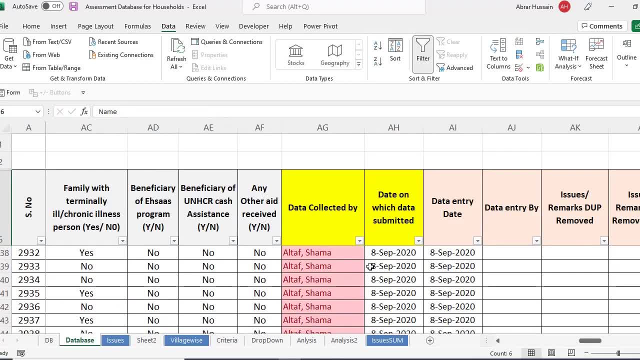 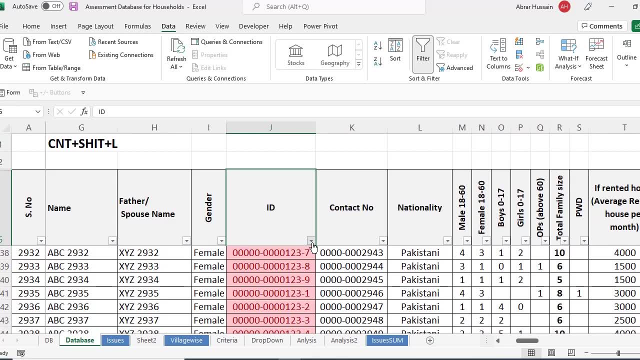 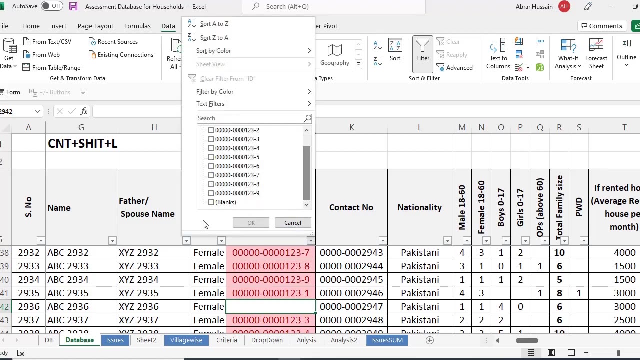 under id. let's check it. this is the id column. okay, here let me see by filtering. and yes, there is no blank information. for example, this one is not here, it is blank, for example. so now you will see and check this and see there is a blank. and now let's go to the calculation. 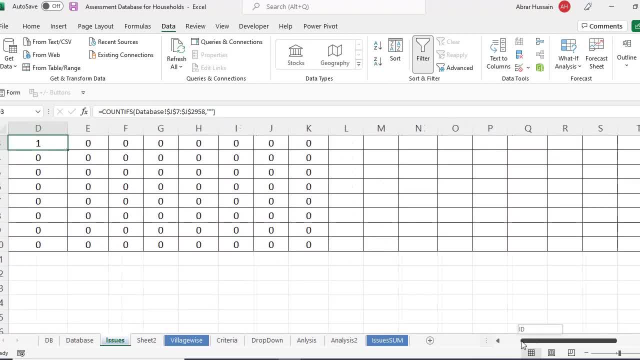 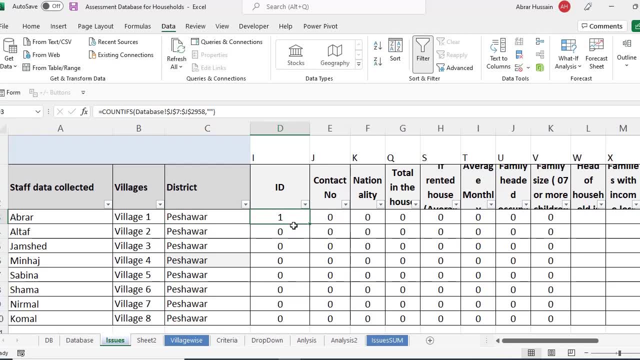 there also. you see there is one digit. it shows that there is one blank information. so whenever you want to see to count blank information in a cell, the simple formula is count ifs. go to that sheet, range that column and after comma say add. these quotation marks are inverted commas. 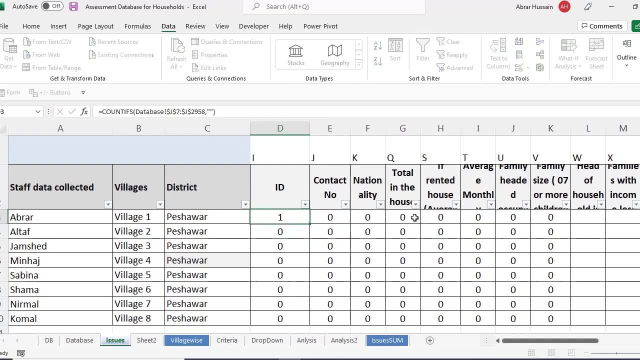 and enter, so it says that there is one id missing. so in this way you can apply this formula to each column and see whether there is any blank information or not. i have written these columns names here. why? because here i just did it with column j, so onward the columns are same, so here i would select. 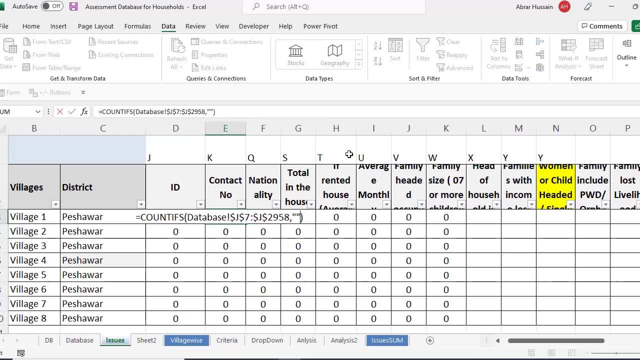 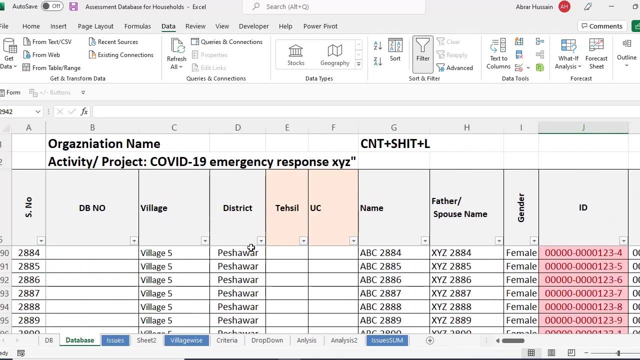 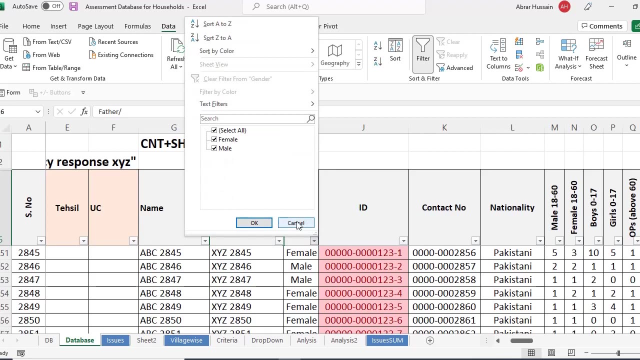 this same formula copy paste here and just say: check it, column k. so there also there is no missing information. so all these you can check. you can also check other ways, for example blank information. then you see by male, female if there is any missing entry in the gender column. 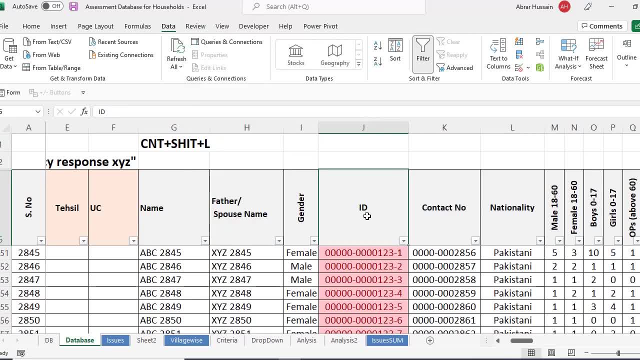 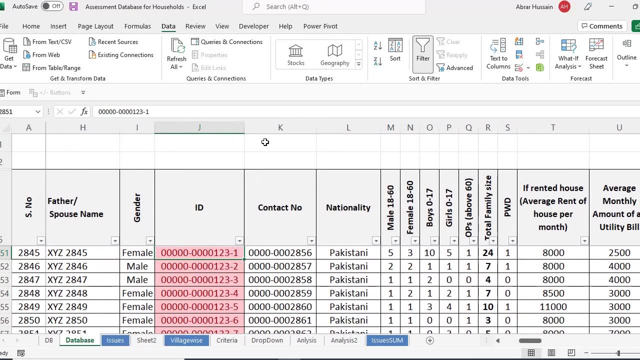 if it is an id card, so, and if it is in pakistan, so in pakistan we say that the last digit of uh id card, if that is even so, it is female, and if it is odd, so it is male. so you can apply a formula here, you can insert a column and you can just extract what is the ID card in your ID card column. 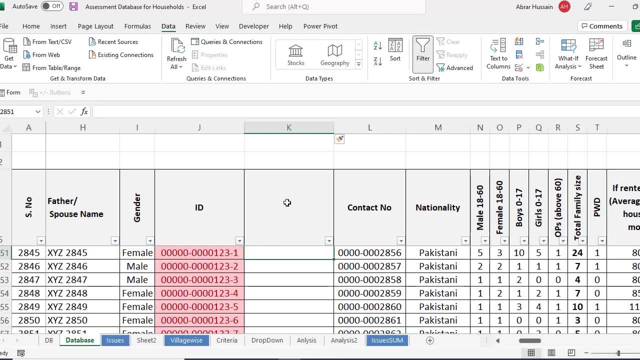 the last digit from this column so that you may be able to filter with. you would have only zero to nine digits in this column. then now here, if you want to filter, you would have a lot of CNICs or ID cards or any number, so you can extract the last digits from here if there is any such. 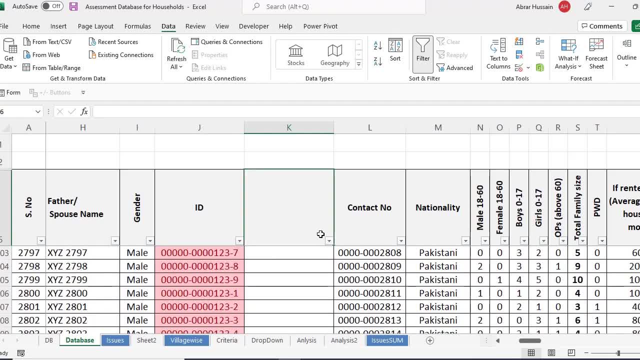 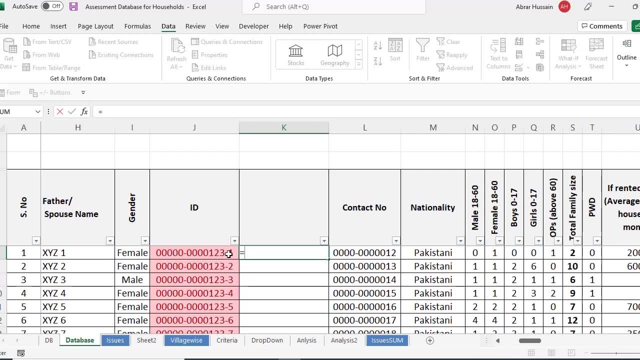 legend available what you can do. you can say what is the formula to extract right side or left side digits. so this one, this one is on the right side, so I would say: right, then I will range this and after comma I will say: one one means the first digit from the right. so it gave me one. if I paste. 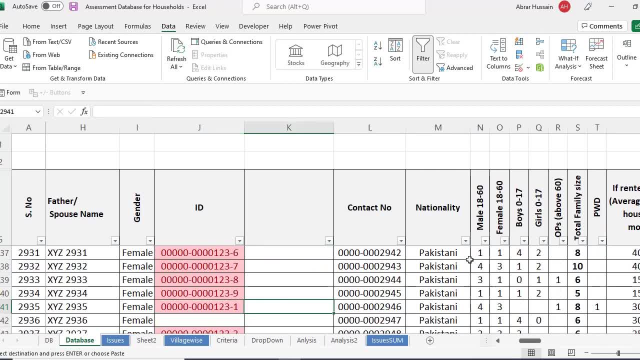 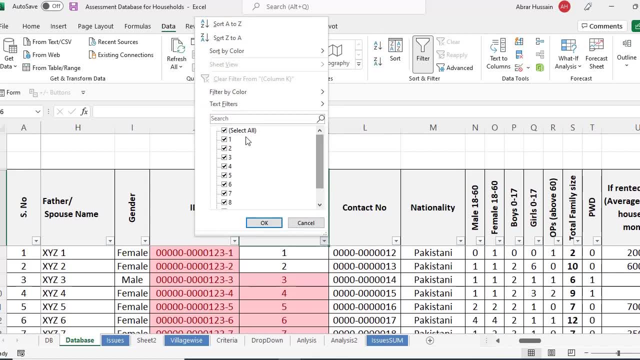 it here. so it will say two and then two and then two and then just drag it. now, here you can see filter in the filter. now you would have only these options. so if I want to filter male one, three, five, seven, nine, select them and see here in this column if 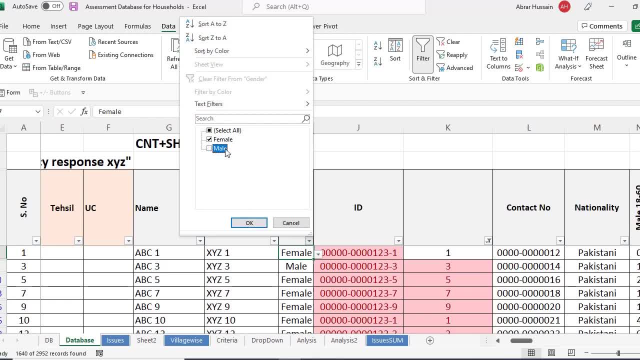 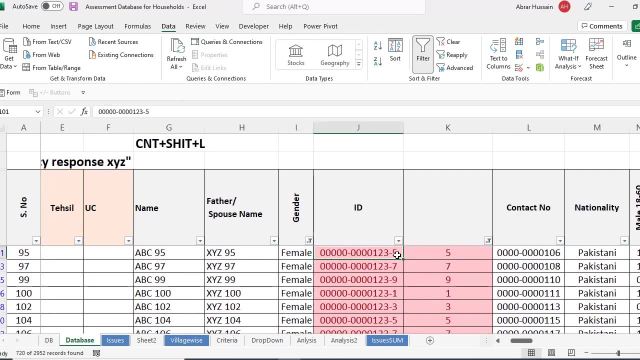 now there is any female so it would be wrong. so I am unselected the male and just selecting the female criteria and applying. so there are almost 720 records whose last digit of CNIC is odd, but still those are female. but it's female just because this CNIC number. I just inserted dummy numbers. 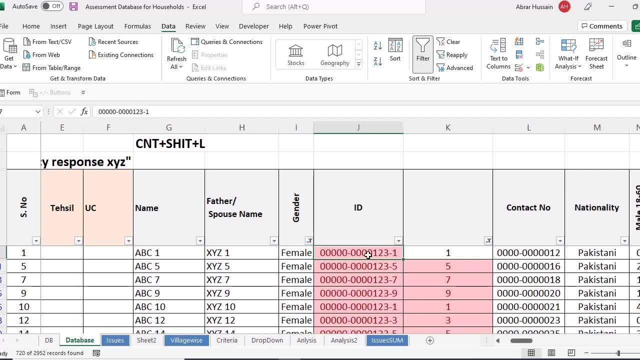 that's why I have just dragged it: zero, zero, zero one, two, three. so you have this option also that if you don't have any gender column and you want to add and you want to add a gender column, then you have to add a gender column and you have to add a gender column. 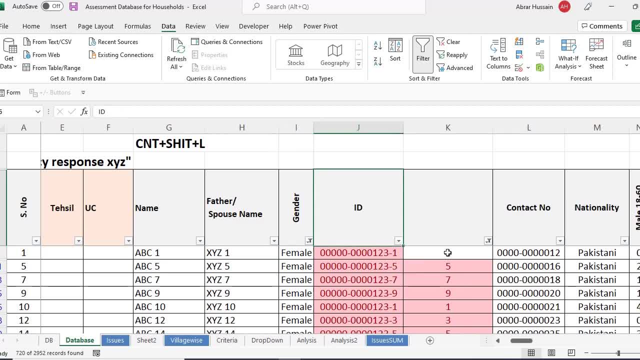 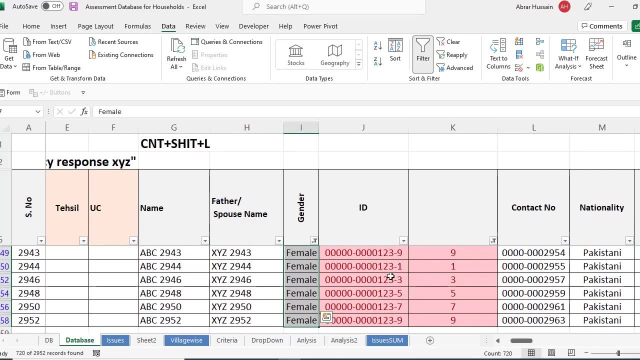 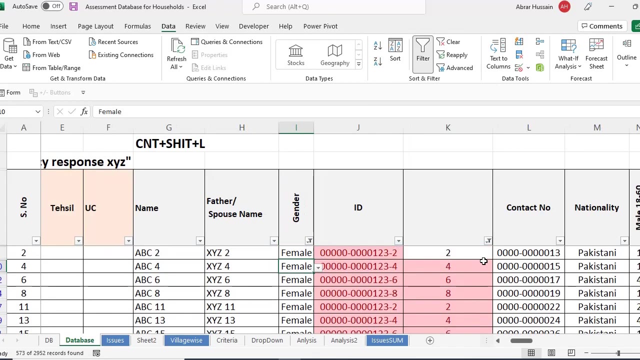 and if you have a ID card column, so you just extract this information and filter all odd and just apply to them male and then filter all female, all these numbers four, two, six, eight, and if there is zero, and mark all of them as female because maybe they have identified a gender. and if they have, 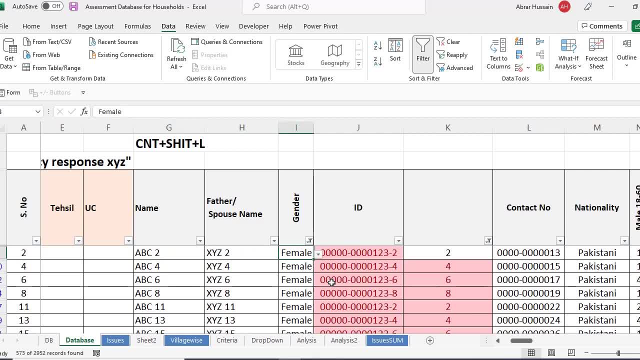 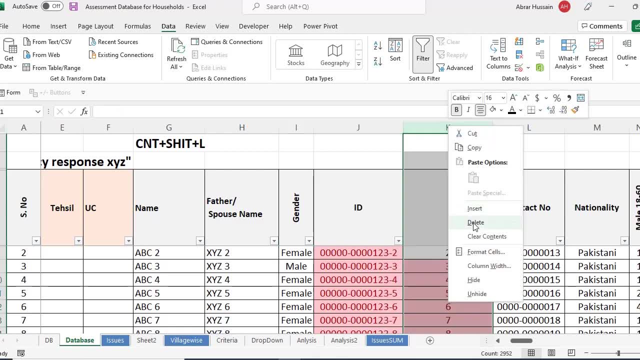 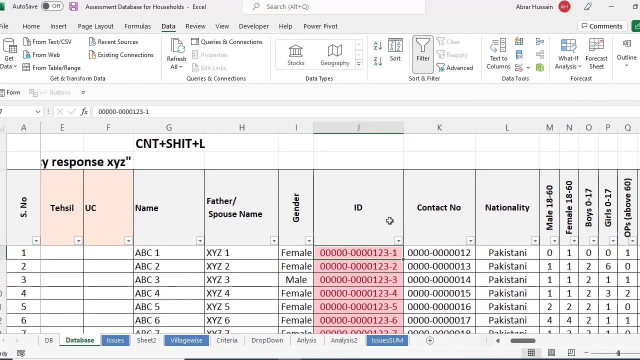 identified a person and by names. it is difficult for you to tell you with the gender column. so that's why you this way you can clean it easily and then, just when you are done, delete this column and other issues that you want to clean. for example, the length of an ID card should be 15. 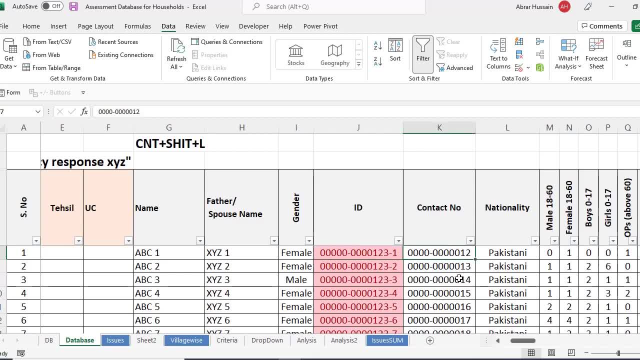 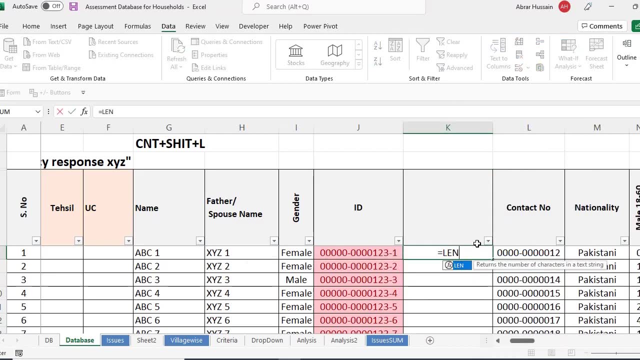 digits in Pakistan, another country, it could be different. and the contact number should be 10, 11 digits, another country, it could be 10 digits. in Pakistan, another country, it could be different. so for this also you can apply a formula. you just add a column and bear is a len formula, Lin later. 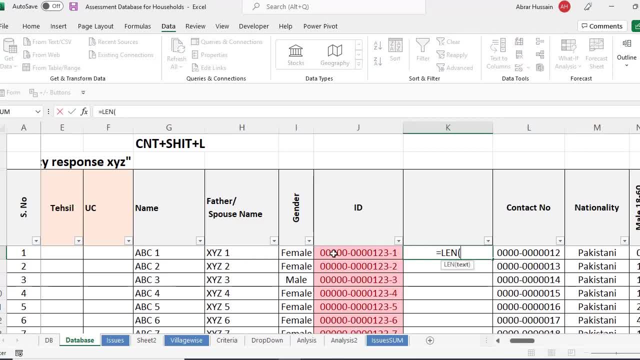 what it does. it found the characters, let how many characters are there in this cell? so I am just applying it and selecting, and now what it shows? it shows 15. so this is correct one, and now I just copy and drag it up and add it and hide it. 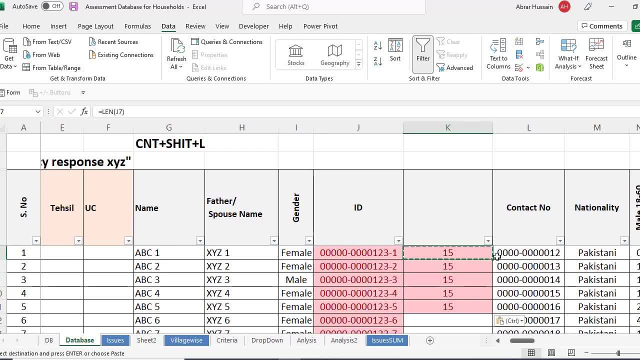 it till the end and then through filter i can see that if there is any digit other than 15, so that cnic would be wrong. so you can easily track that. similar formula you can use for contact number. just add a column and the same lin formula and then arrange the contact number and it will show. 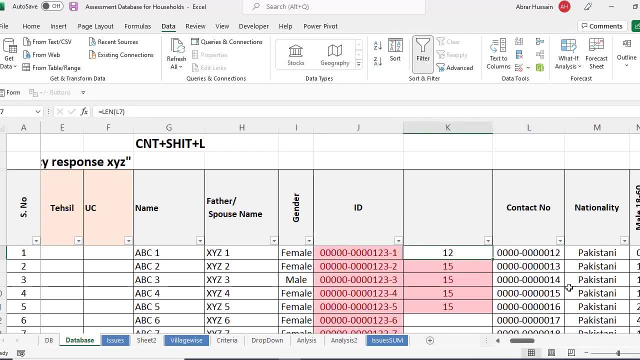 12 digit. 12 digit because there is a dash also. so if there is a dash, then it should be 12, if there is no dash, then it should be 11 or 10.. so you can apply this also. so these two formula, the right. 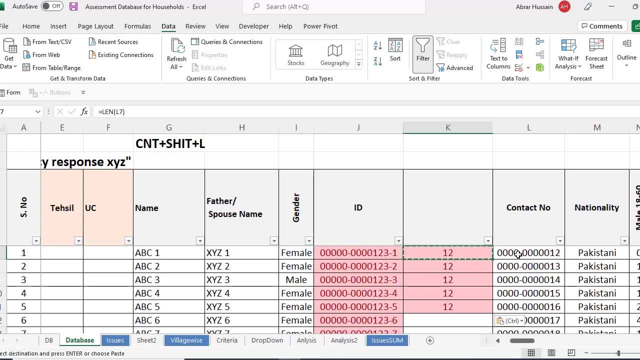 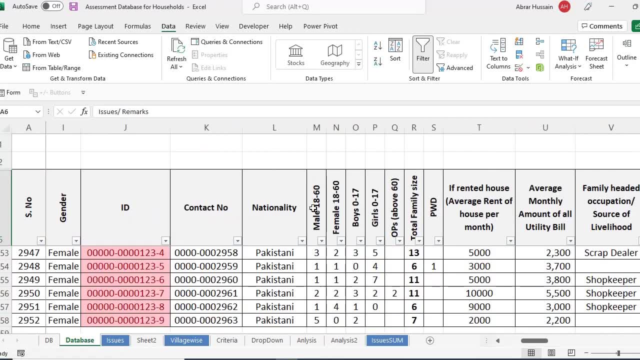 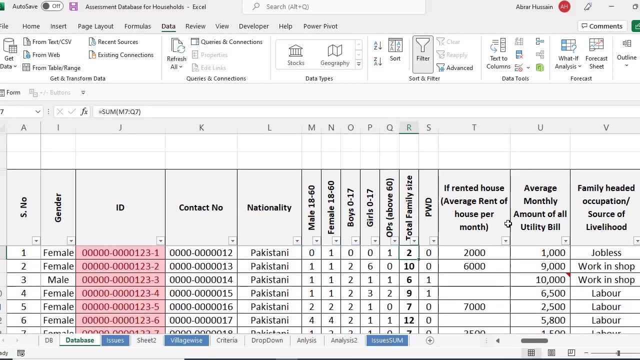 left formula and the l, e and lin formula provide you these cleaning techniques to clean your data easily. other cleaning option for you are also these: you know the number of family members between different age groups, so you can. this one is the total one, so it should be a formula counting all these, some with some. so here also you can just see whether there is. 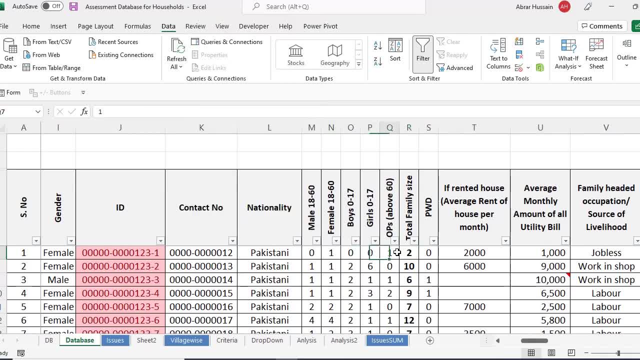 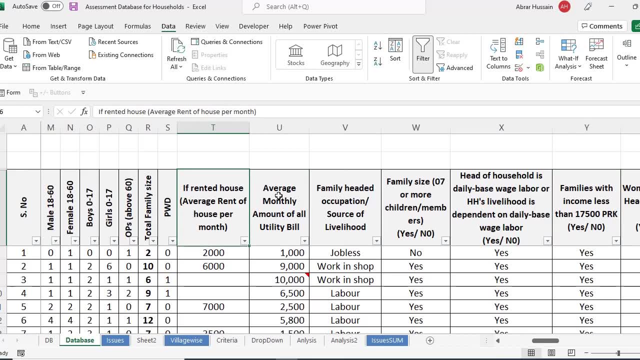 any blank information or something so you can just check. now onward the cleaning might be a little bit difficult because uh, they say if rented house, average rent of the house per month. so if there are blanks so that means that the person house is not rented, simply, but it might. 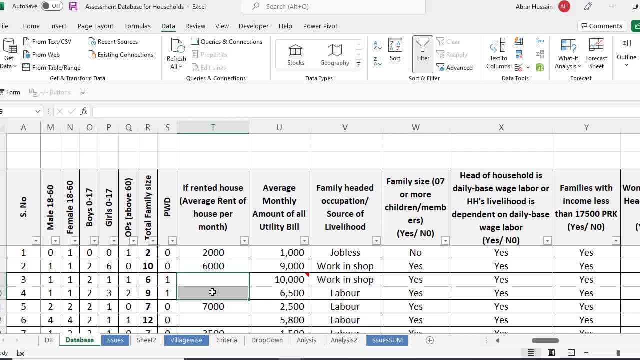 be because they have not provided this information or the data. the person who was collecting the data has not added it in the form, so that is also a difficult thing to you know, identify, and for that you would need some you know follow-ups- uh, sample based follow-up with the beneficiaries, for example. 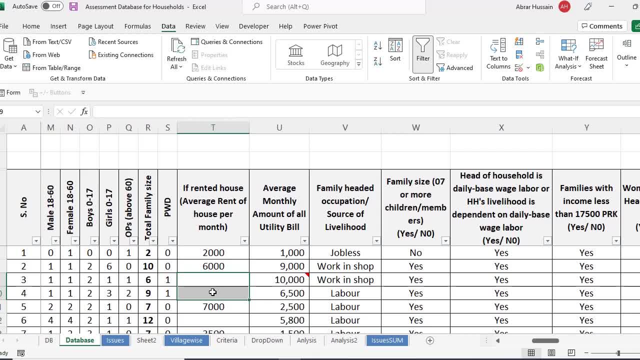 say you have 5000 record, you just select 10 percent of the sample and just call them and verify these information so that you may have authentic information. average monthly amount of all utility bills. here also you can check some um you know, for example, if there is any. 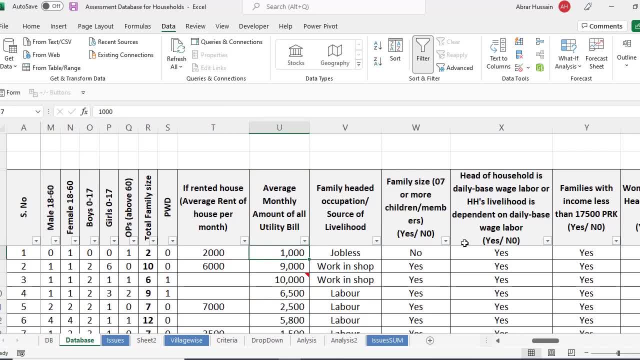 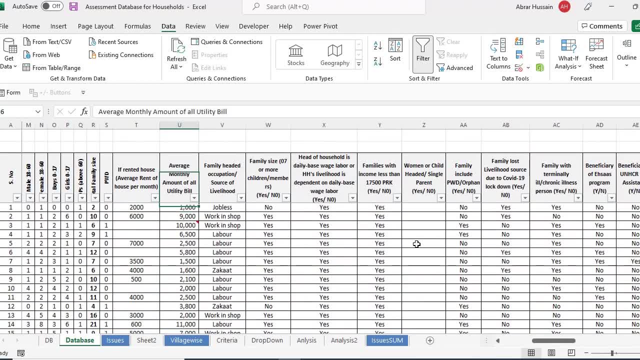 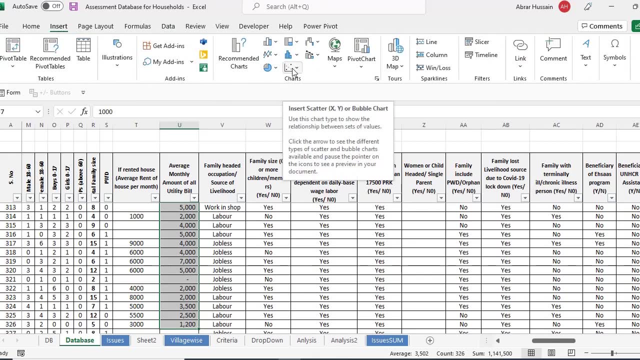 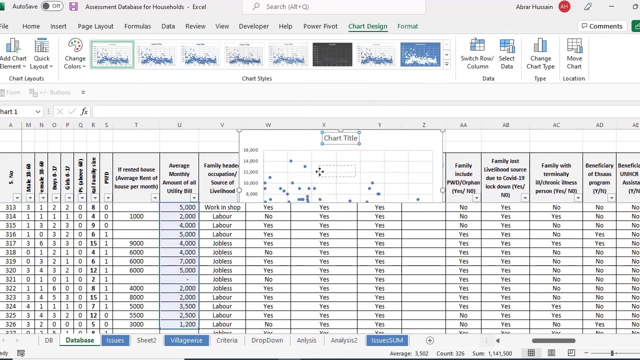 number that is totally out of the range, as we say, data outlier. so you can just do that for the graph also. you can develop a graph. just select this whole column, go to insert with this also: this is x- y scatter- x- y- scatter. this do what things you see. now let me explain this, this chart, to you. 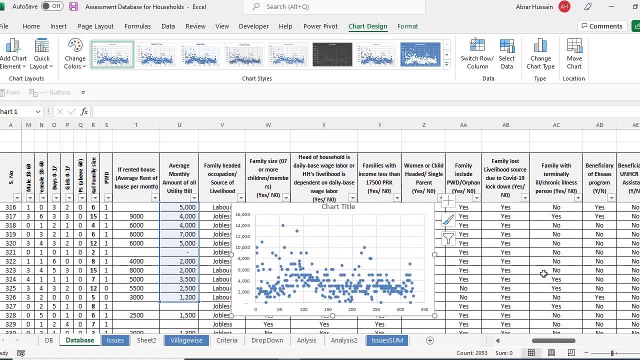 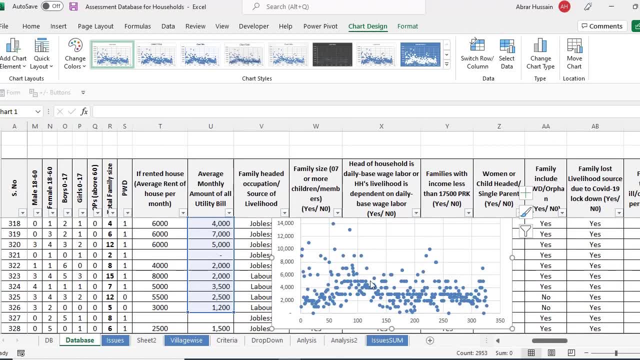 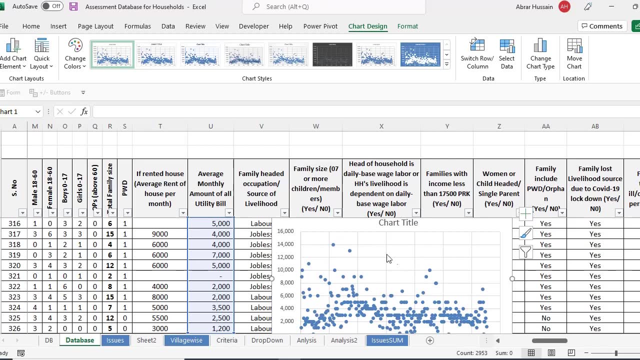 in this column if you want to see any abnormal data. for example, if you look at this chart, the data is here, but if you see there are some dots which are far away. you see there are some dots, so you can identify these, but this chart only gives you the idea that. is there any anomalies in? 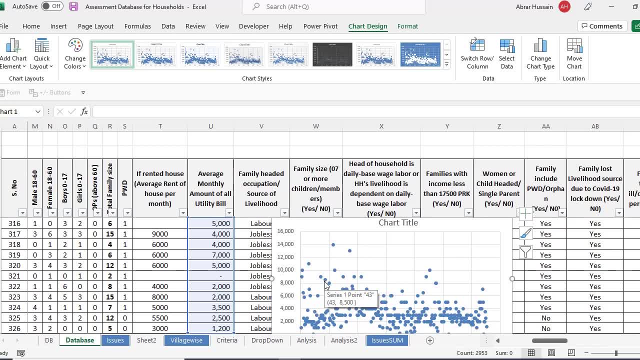 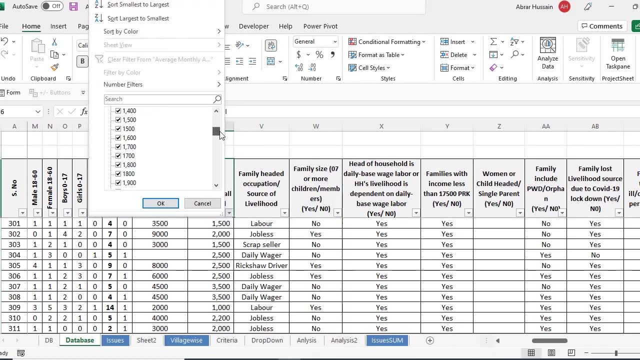 your data or not are in is. are there any outliers or not? now, if you know that there are some outliers, you just go there. you see there is 0, 100 and there are 8, 45 000, 4 000. now you can filter these information. that why the utility bills of such vulnerable communities? 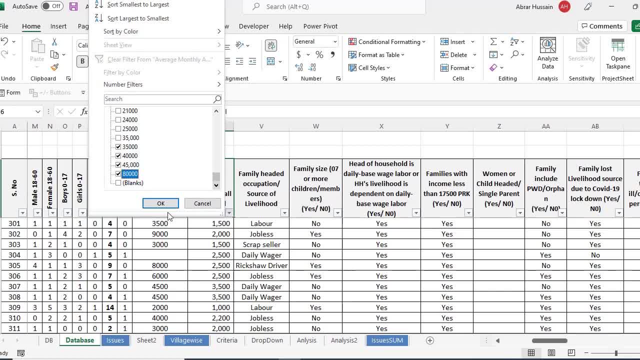 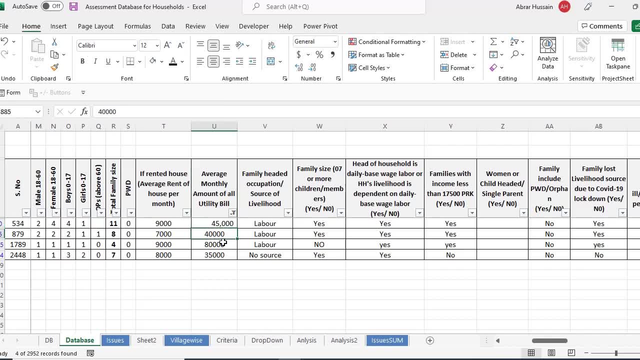 to whom i am going to give some support. what's so high? average monthly bill of a person is 45 000, 40 000, 8 000, 35 000 and you see the occupation of the. how is it possible, so you can identify. 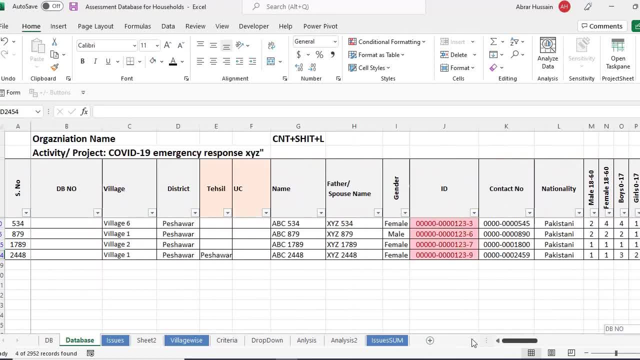 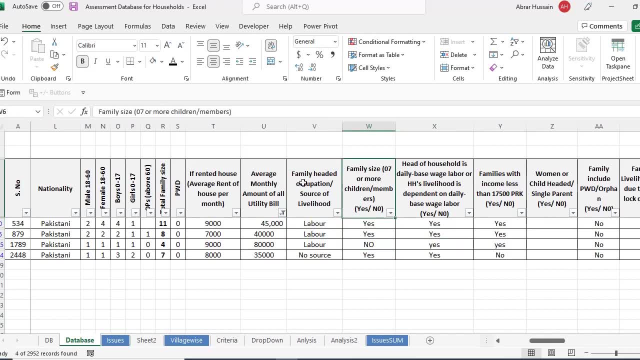 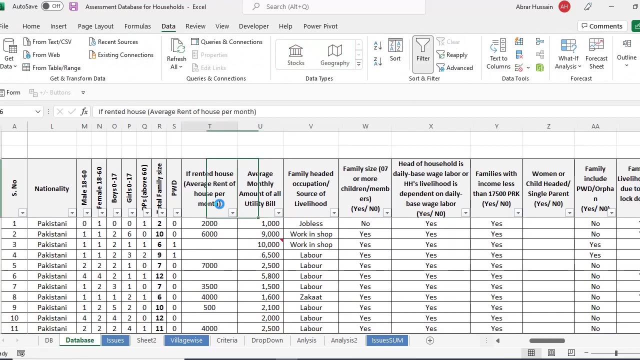 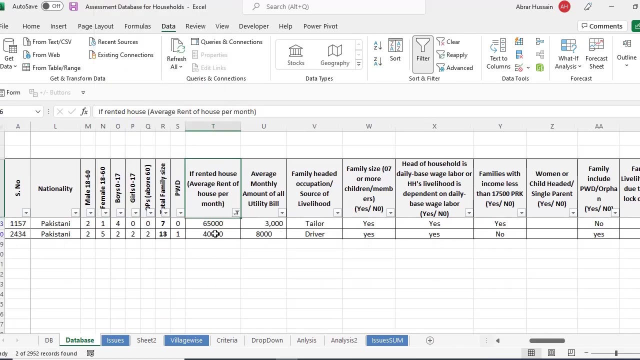 these outliers so you can identify these different types of uh anomalies in your data. in this way, because you have most of the information available, so you can clean it- you can see whether a rent of a person is higher than, for example. see these two people: their average monthly rent is 65 000, you see, and the next one is 40 000. 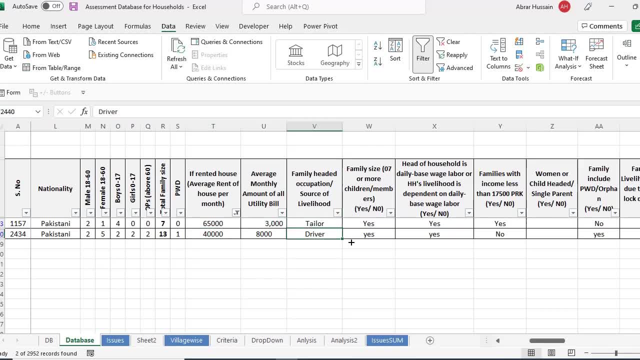 and the person occupation is. you can just verify these things. so when, uh, you are going a sample based verification, so you can do this by this. well, so that all the records where you find such issues, so you can call them and in confirm the information from them also, and in this, 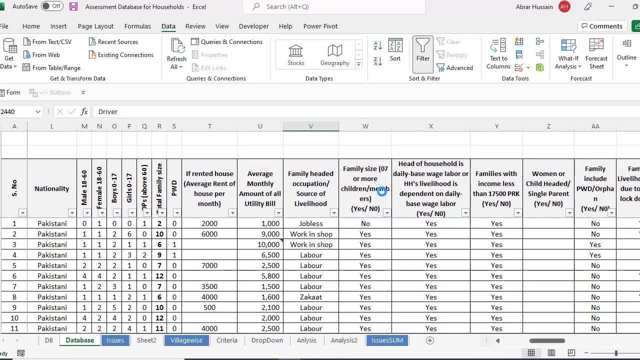 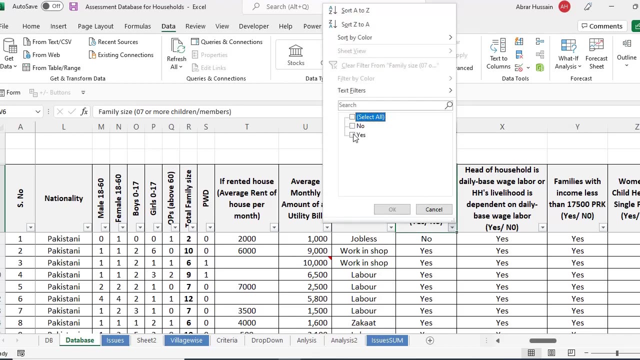 you can use different strategies, different ideas to correlate different columns, data and see whether there is any missing information or not or any sort of issues. for example this: this column says whether the family size of the household is 7 member and more than seven member. now, for example, i filter here all those who says yes, their dear family size. 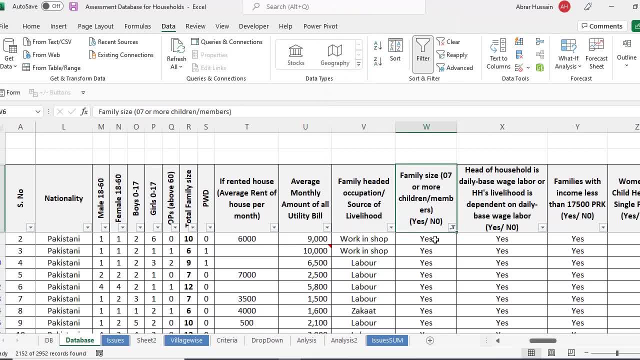 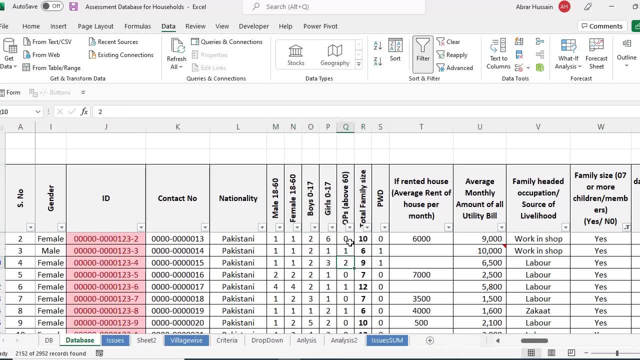 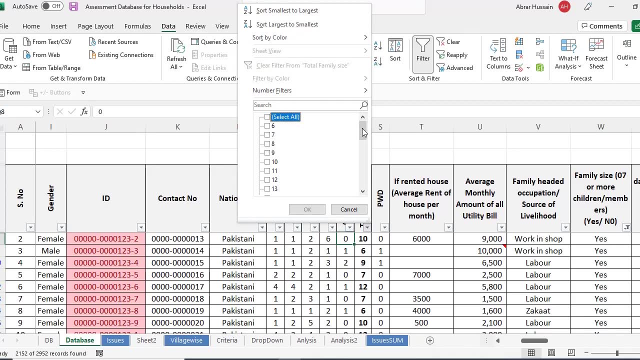 as more than seven. so I have filter all yes. now just look at this column where they have provided us the number of people living in their home, so you can verify with these also. now, here you see there is one family with six members, but that's okay, he might have not counted himself, so you can just you know.